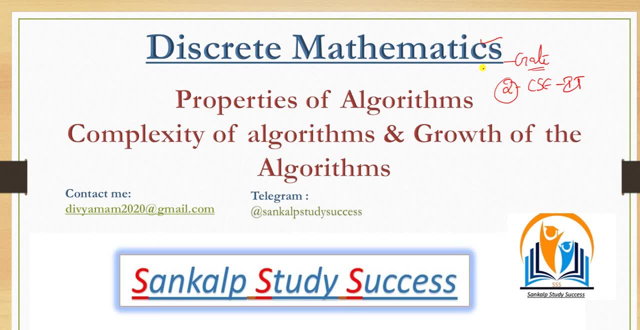 So in discrete mathematics, not only topic wise, just I want to discuss unit wise, okay, So some set of concepts will be there in every unit. So now today's session I am going to discussing about unit 3 in discrete mathematics. okay, 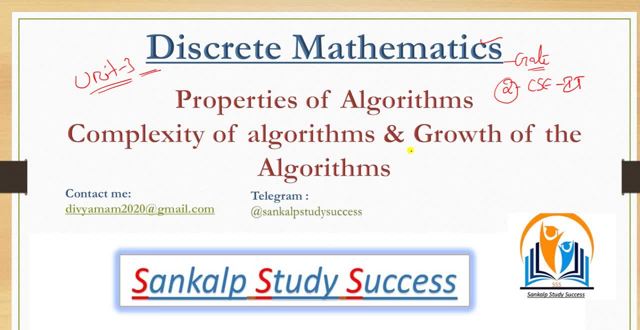 So in unit 3, we have a properties of algorithm, complexity of algorithms and inductions and recursion Clear. So if you have any doubts, please message me. divyamam2020 at the rate, gmailcom. This is very, very important subject for GATE purpose. 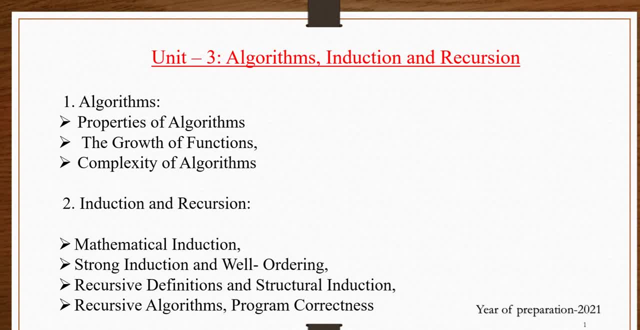 See here in the unit 3, we have all these concepts: properties of algorithm, growth functions and complexity of algorithm, and inductions and recursions, In that mathematical inductions. this topic is very, very important, okay, So let us discuss first one: algorithms. 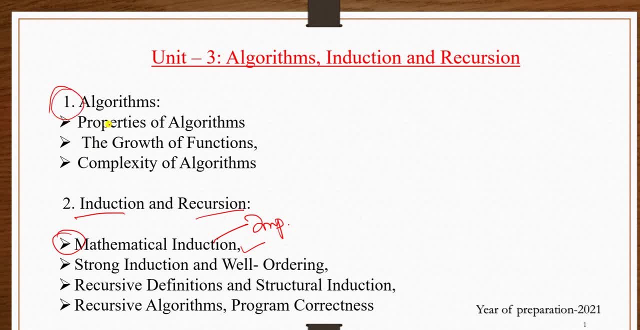 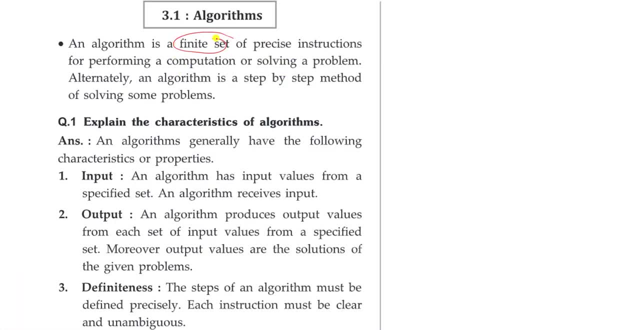 The first part of so In this session I am going to discussing about the first part of third unit. Clear Now see what is algorithm. Algorithm is nothing but finite set of precious instructions. Means a step by step procedure. 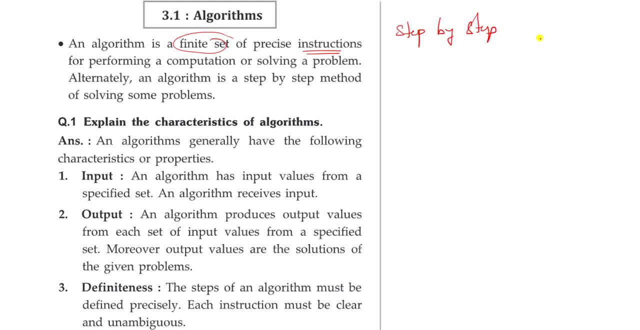 A step by step procedure. Let us take any example or any program or any method. Okay, What we have to do? We have to follow the step by step procedure. Then only we will get certain output or correct output, Right. So that particular step by step process is nothing but. 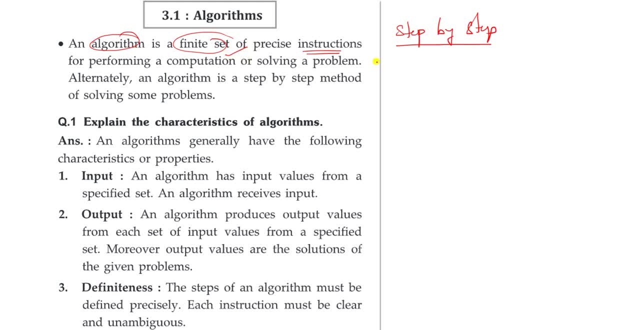 Algorithm, Okay, It is a finite set, not infinite set. It is a finite set. Remember this Very, very important: Algorithm is a finite set of instructions. These instructions are performing the computations or solving a problem, Okay. So alternatively, we can also say that algorithm is nothing but step by step procedure to solve the problem. 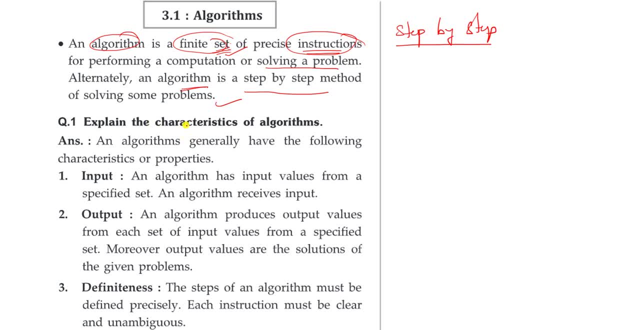 Okay, Next come to the next topic of algorithm, That is, characteristics or properties of algorithm. So generally, In algorithm, Algorithm, we have several characteristics and several properties. So here we have seven properties actually. So what are the seven properties, or input? 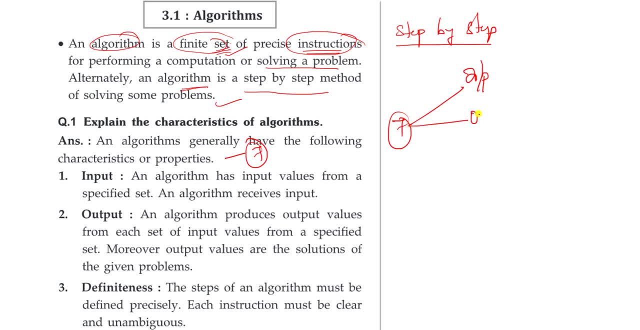 Here IP. IP means input, And finally we have the output: Okay, And finally we Next one, we have definiteness. And next we have correctness: correctness, finiteness, effectiveness, effectiveness- Okay, And next one, we have general. 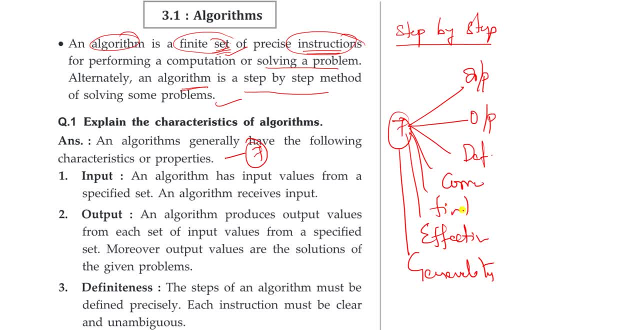 Generality, Okay, Generality, So these are all the finiteness, this one correctness, this one, Okay. So these are all seven properties we have for algorithm. Okay, So in order to write an algorithm, you need to follow all these properties. 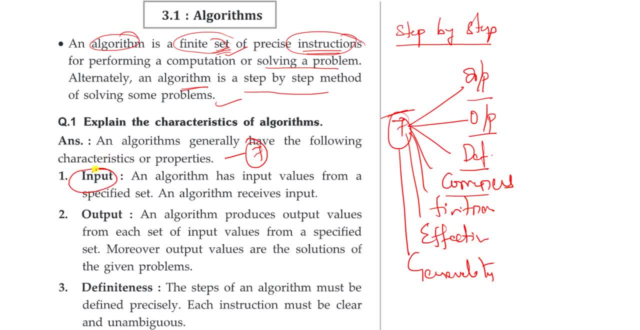 Now see the first one by one, What you mean by input. You see, as you are a engineering students, that too: CSC and IT, Okay. So mostly you people for software works, So you will learn about Okay. 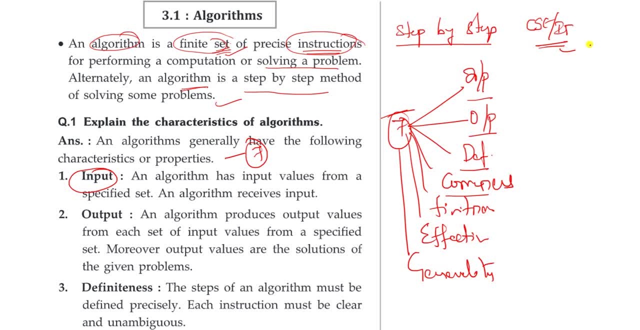 software jobs only you. you will do only software jobs right in software sector. you have many platforms, many languages are existing in that. so before going to writing a code for a particular project, what you have to do- you need to write an algorithm for that particular program before going. 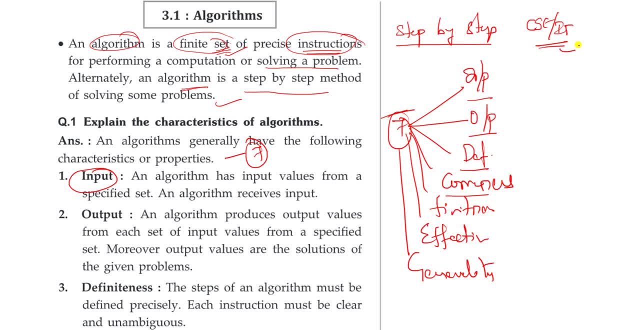 to write a core code, you what you have to do, ma you have to write an algorithm. that means step step process. what are the variables we should use? what? what is the main theme of rls? what is the main problem of that program? okay, how we consider it. what next? what we have to add, what we have to. 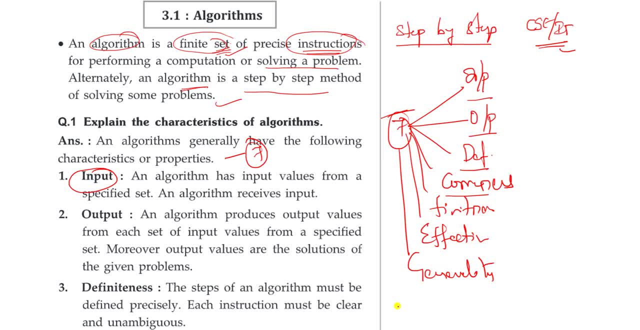 subtract or what we have to search. likewise, that is depending on the program, depending on the problem. we have to write the steps in algorithm, right in that. first thing, what, what property we have to check you, input, input here the values that are from the specified set. so what? the values that gives to 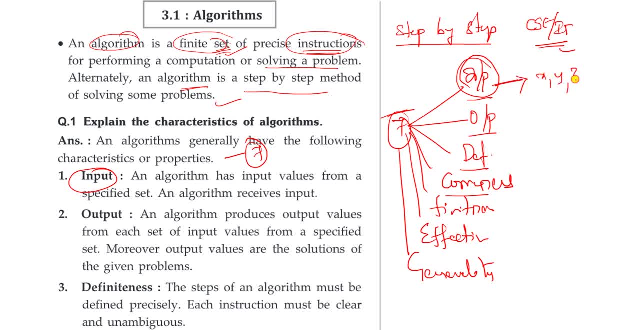 the algorithm is nothing but input. let us take some x, y, z variables. so these are all the input values. so here algorithm has an input: values from specified set ma. so here algorithm receives output. algorithm which receives the output and it gives the out. sorry, it receives the input and it will. 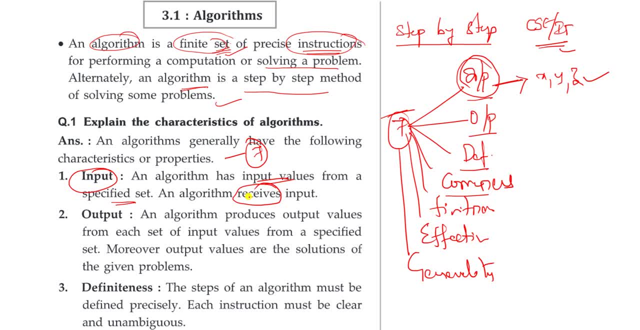 gives the output clear. i repeat the statement. so here an algorithm which receives the output and it will gives the output. so here an algorithm produces output. that means it gives the output values from each set of the input values from a specified set. so here me again, japan. new input means what? uh, it receives the input values from 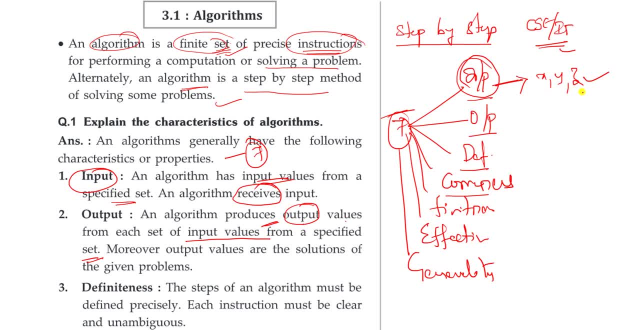 where specified certain in depositive했던 d, and it will give us the orden, or else it will produces the output. it will produces the output. for example, z is equal to x plus y. okay, so after addition of these two variables, the particular variable, the particular answer that will shown. 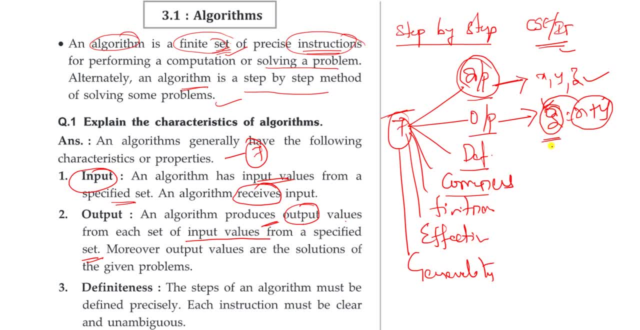 on the z value right. so here the output variable will be z, right. so, moreover, here output values are solutions of the given problem. so what is the output here? our solution. and next one, next property is definiteness. definite means here the steps of algorithm must be defined previously. 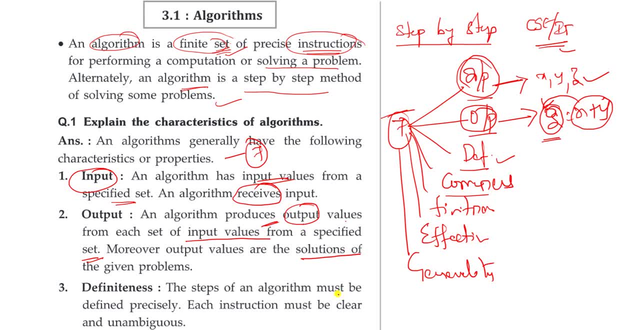 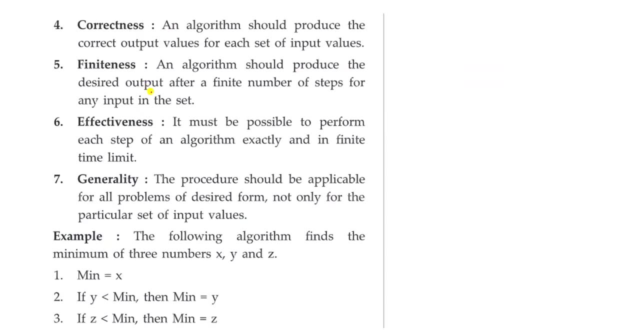 each instruction should be clear and ambiguous, ambiguous, clear. so every instruction should be clear, okay, clumsy, clumsy, it should not be clumsy. each and every step in algorithm should be clear and ambiguous. okay, and next one: correctness. correctness means what it should be: produce a correct output, values. it should not give the wrong output. that is correctness. 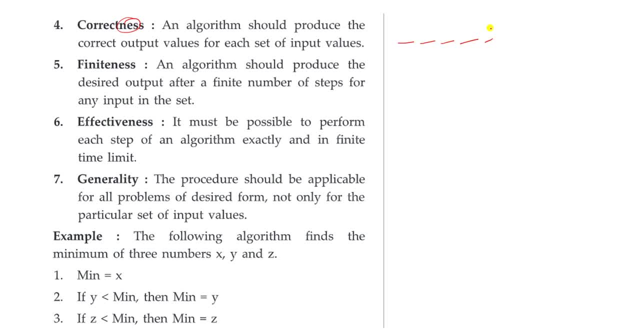 so after doing all the steps in algorithms- for example, let us take one algorithm, one and not only brackets. we have several steps more okay around. my steps will be there. after doing all these steps, you have to get the correct output. for example, let us take x comma, y comma, z values: x is equal to ten and y is equal to twenty. 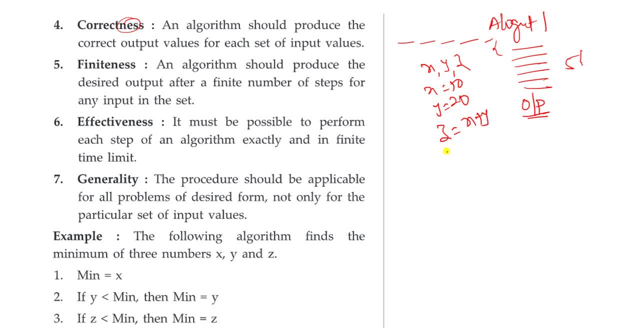 and here what me on? z is equal to x plus y. okay, so we want to do addition of two values. z is equal to ten, is equal to variables, so after that we have to get the output value. so what is the output value for this? what is the z value? 10 plus 20, that is 30. okay, we should get 30 value, because this is the correct. 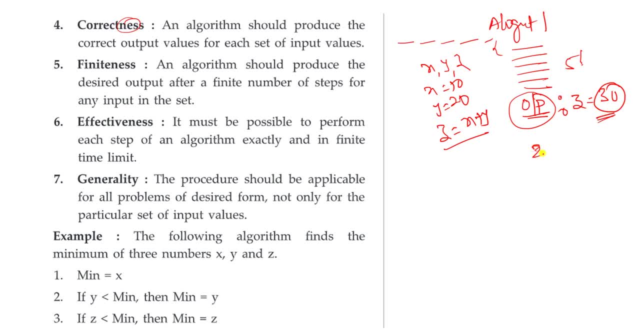 output. we should not get other than 30, like 20 or 10 or any 50 or any 70 value. because of these two variables, 10 and 20, we should get 30 only. that is correctness of algorithm. after doing all the steps in algorithm, that particular algorithm should produce the correct output values only. 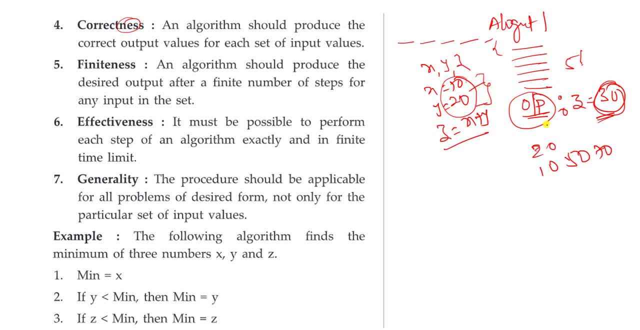 for all each input set values. these are all the input values. this is the output value. okay, and next fourth property is finiteness. finite means it should be finite value. finite number of steps will be there. there is no infinite steps. okay, here let us take some five steps, or seven, seven. 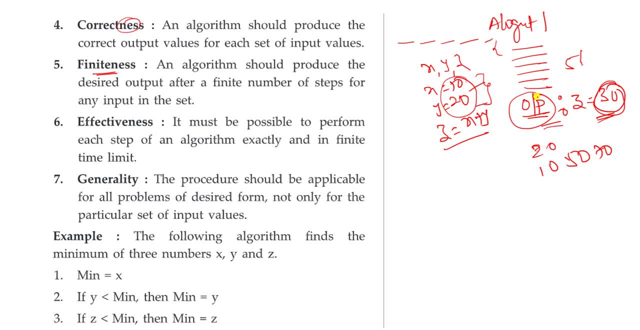 steps, or ten steps, or all hundred steps. finite number of steps will be there in algorithm, okay, okay, in an algorithm it should produce the desired output after a finite number of steps or any input in the set. so here, what, how many steps? we have one and two, three, four, five, six. so here we. 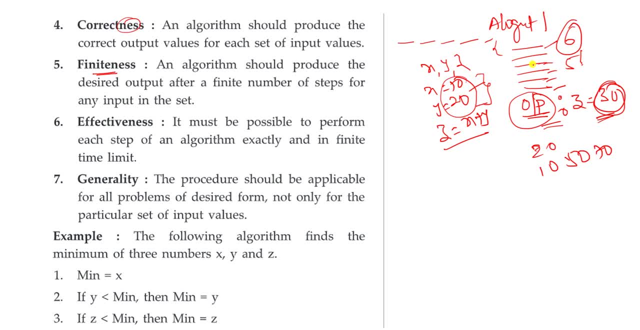 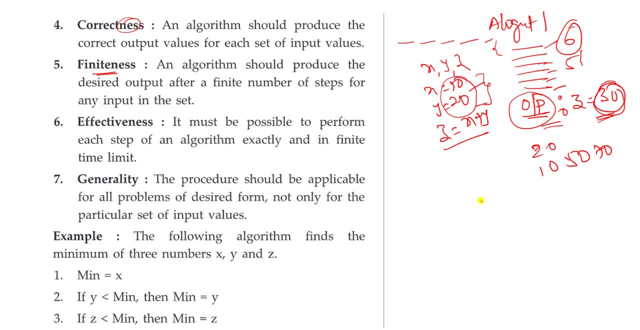 there. what will be happen? you did not get the output at any time. okay, the program will be going, going on. it will be run next. effectiveness. effectiveness means it must be possible to perform each step of algorithm exactly. and infinite time limit. okay, the prescribed time limit will be there, within the time limit only that that particular algorithm will be able to perform. 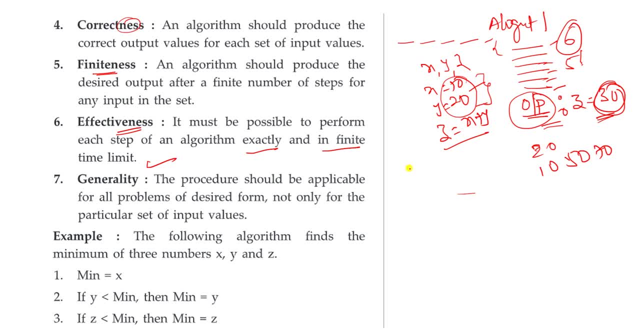 the algorithm have to be um run. okay, that should. that is nothing but effectiveness. and next, generality. generality means applicable for all the problems of desired form. okay, not only for the particular set of input values. so here let us take um. uh, i wrote some algorithm for addition of. 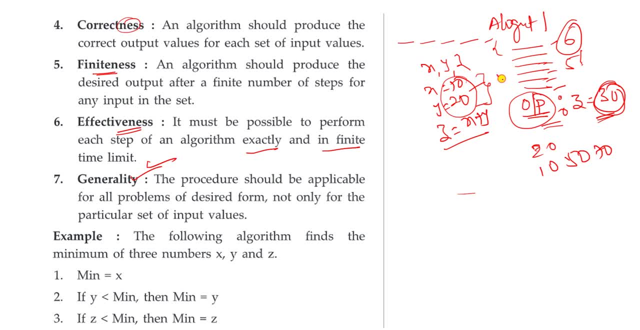 two numbers. okay, so here this particular algorithm is available for all problems of desired output. okay, not only for x equal to 10, not only for x equal to 10, but for all the problems of desired output. okay, not only for y equal to 10. you can take x equal to 30, y equal to 40, so you have to follow. 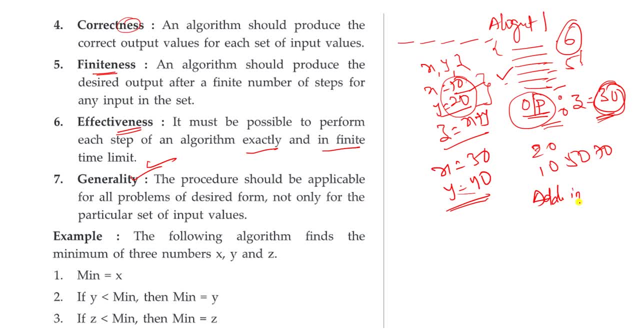 the same procedure, that is, in addition in uh, addition of two variables in algorithm. right, hope you understand generality. generality means applicability, applicability, this particular here, this code is um. what? what is this code? this uh, what are the steps in algorithm? one addition of: 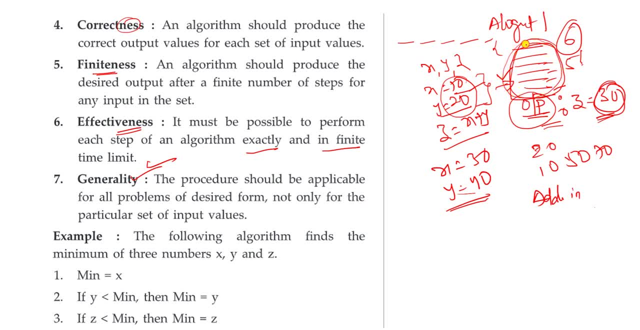 two variables so you can take any input values, this particular algorithm will be used. okay, no need to write again. this is not only for the particular set of input values. that means this is not only for 10 and 20. you can take x equal to 30, x, y equal. 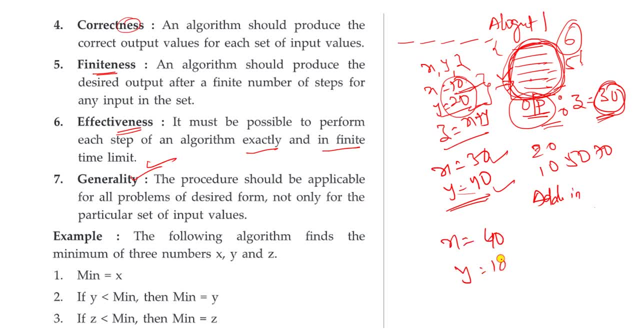 to 40, or you can take x equal to 40, y equal to 100. okay, so 40 plus 100. what is the z value? 140? so here 140 is the correctness, correct value, clear, ma. so that that is about we have several properties. 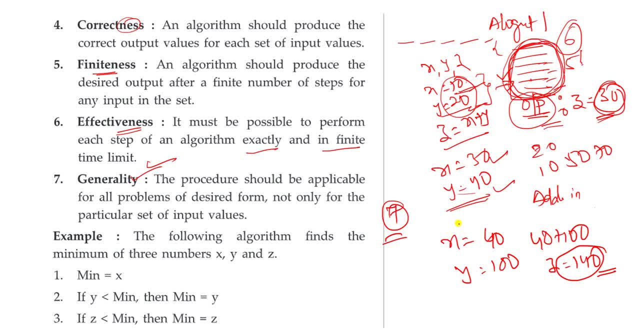 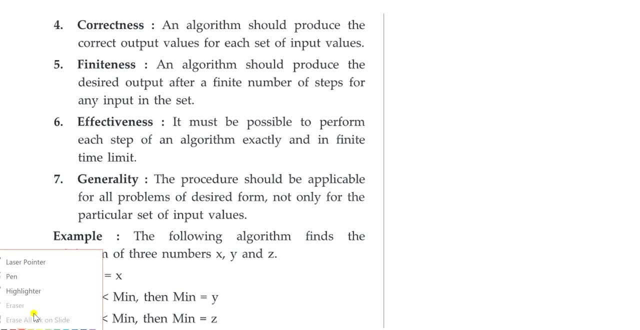 in algorithms: input value, output value, finiteness, correctness, finiteness, effectiveness and generality. okay, let us see the example here. algorithm finds the minimum three numbers: x, y, z. so see the example here. minimum e, let us take minimum value- is x. what is the minimum value? so here, how many variables? three numbers: x, comma, y. 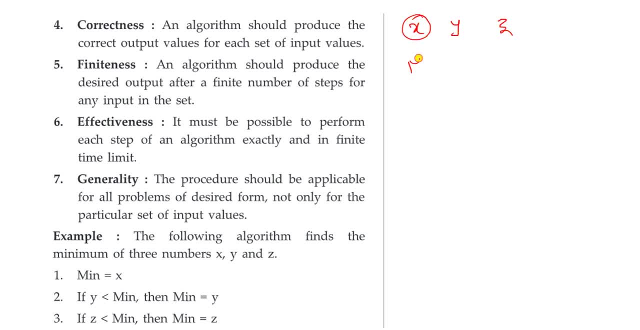 comma z. first let us take that minimum value is x, so here algorithm will be: in the first step, in this algorithm, minimum equal to x. okay, then second step: what we have to check whether second variable, that is y, if y less than minimum. okay, let us take. 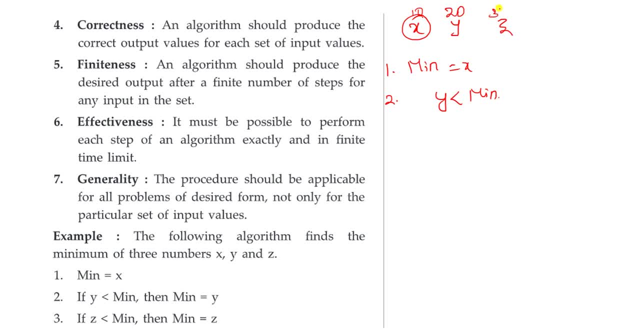 x equal to 10, y equal to 20 and z equal to 30. okay, so here: minimum equal to x. that means what is the value? minimum equal to 10. now check the second value with minimum value. so what is the minimum value? that is 10. so here, what is the y value? 20, 20 less than 10. is 20 less than 10? no, now go to the 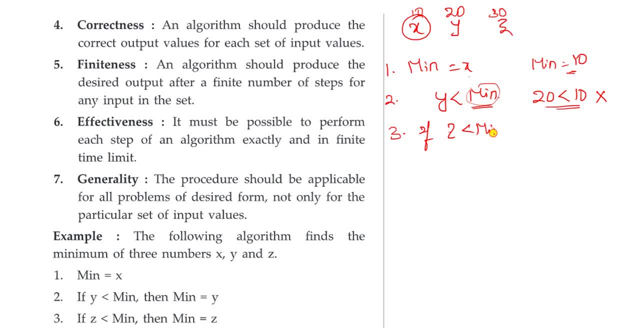 second step: if, if z is less than minimum, what is the z value? 30 is 30 is less than. what is the minimum value 10? no, so y is not a minimum value, z is not a minimum value. so what is the minimum value here? x value. so print: 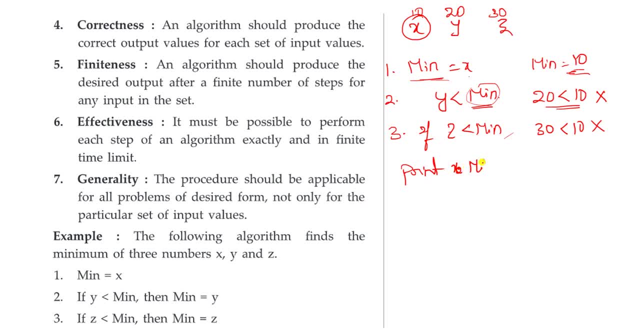 x, simply print x. that is print minimum, right? if for example, here, y value is 5, let us take 5. y value is 5, okay now. now here what we have to check. in first step: minimum equal to x, minimum equal to x, that is, x value is 10. here x value 10 comma, 5, comma 20: okay. in the second step we have to check: 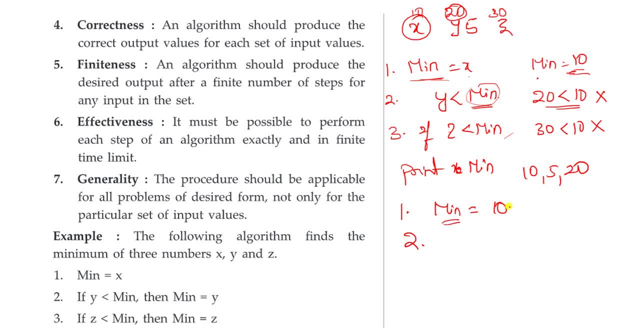 y less than 10 or not y less than minimum. here y less than minimum, that is 5, is less than 10. yes, then print y, then print y. that means what is the minimum value? 5 here. now, what is the value there in the minimum? 5, not 10. okay, it turns to 5. now again, check the third value, z value if z. 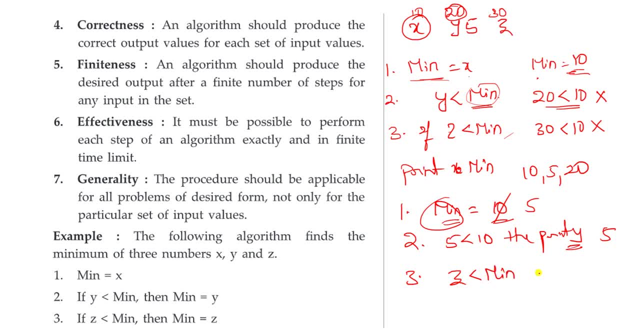 less than 10. z less than minimum means what here? 5 less than not 5, 20 is less than 5. no, so what is the final value? minimum value? 5 only like like this, we have to find out the algorithm. so simply algorithm, how many steps we have. we have only three steps in this algorithm. okay, so the time consumption. 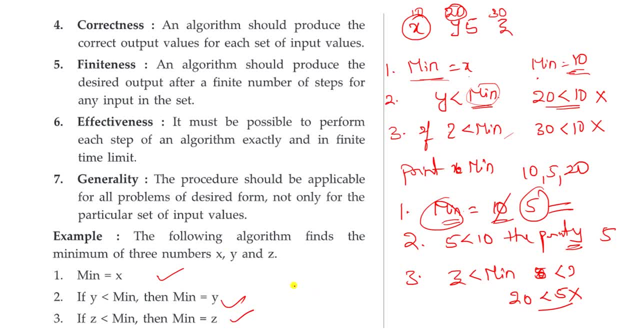 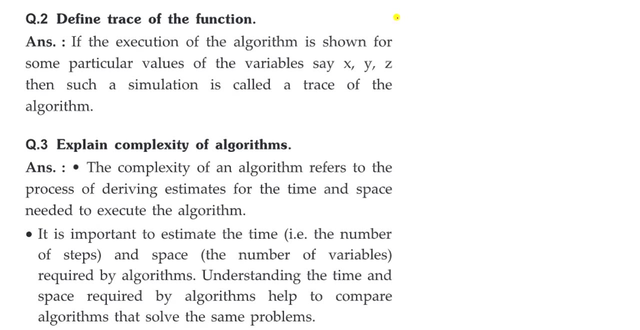 also very less. and also how many steps. we have three steps only, right, three steps only, so finite number is there. how many steps? there is no infinite steps. we have three steps, only finite number is there. okay, now, and next concept is define the trace of the function, so define the. 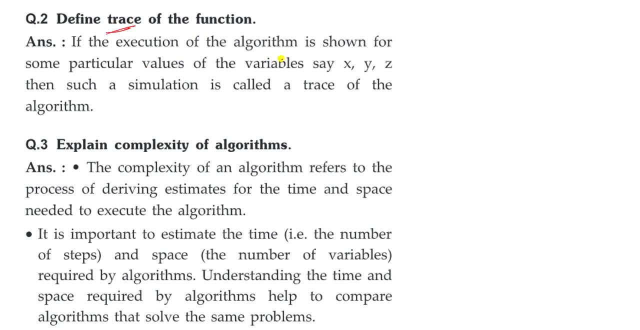 trace of the function means: if the execution of an algorithm is shown for some particular values of the variable, say x, y, z, then such simulation is called. we can, we can call it as trace of the algorithm. what, what does it mean here means we have some algorithm. let us take 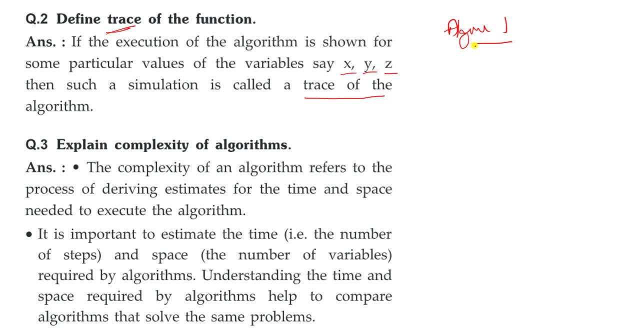 some algorithm one. okay, so this particular algorithm one have some variables. let us say those variables are x, comma, y comma, z. okay, so these variables, some values will be there, some execution time will be there for this particular of these particular variables. so the execution of algorithm of these variables is nothing but trace, repeat the statement, the execution of the algorithm. 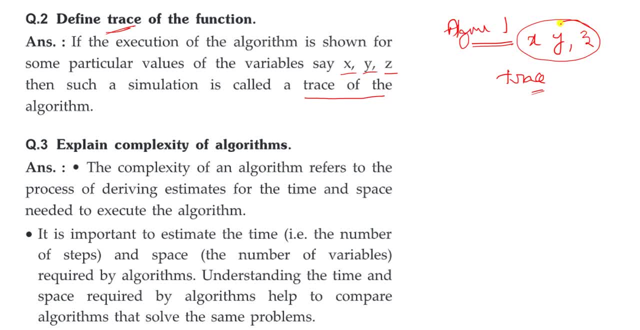 of these particular variables, how, and the entire execution time out on the e3 variables. that is nothing but trace. okay, now complexity of algorithm. so what is the complexity of algorithm? it refers to processing, of deriving the estimation of time And the estimation of space needed for that particular algorithm. so complexity, okay, remember. 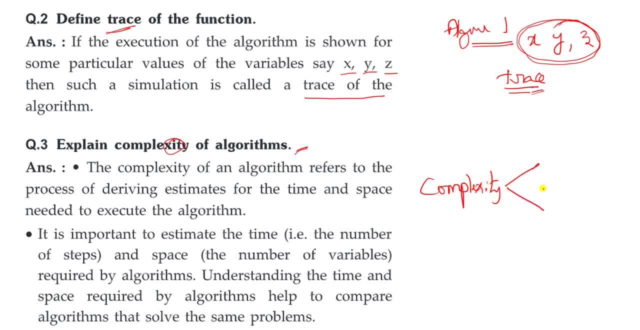 this very important complexity of algorithm. we can determine time and space. okay, we can determine time and space with the help of time. we have to estimate the time here. time in the sense: how much time is required to execute that particular algorithm? okay, how much space is required to save? 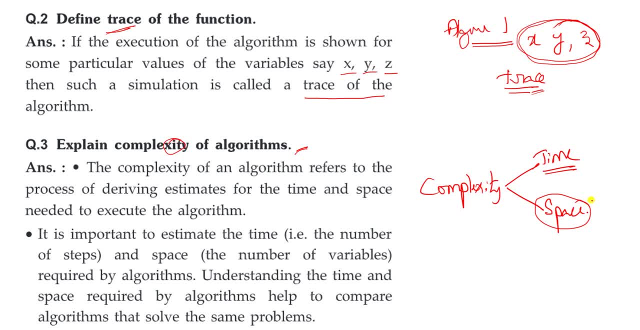 that or to store that particular algorithm In the system. clear. so that is time complexity. time complexity and space complexity, right, so very, very important complexity of algorithm. so it is very important to estimate the time, because number of steps here um time is depending on the number of steps. if number of steps is less in a particular 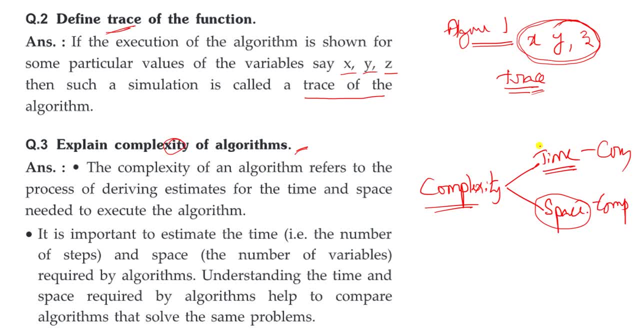 algorithm, then what will happen? um, run of the program, execution of the program will be low. okay, when compared to the more number of steps in, for example, here today, algorithm. let us take two, two algorithms: algorithm one and algorithm two. okay, for example, let us say an algorithm one. we have. 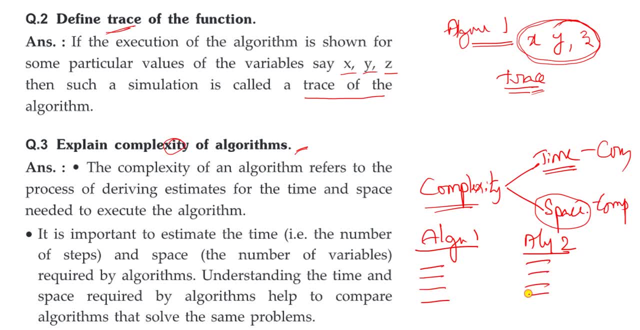 some one, two, three, four steps only. but in algorithm two we have eight steps. okay, so here for algorithm one we have only four steps. so for execution of these four steps, how much time we required for execution of algorithm? we just required two seconds. two seconds of time is required. 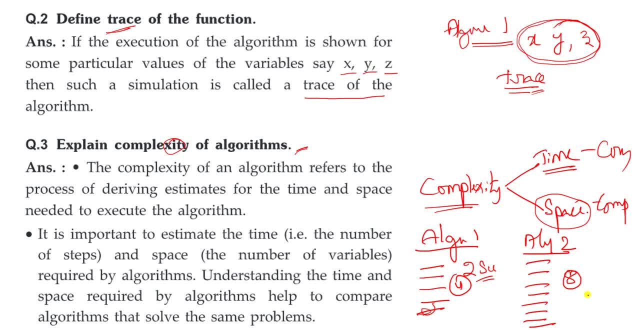 okay, for here we have eight steps. for these eight steps, how many? how much time is required to execute this algorithm to? we required four seconds. let us take just assume this example to so here, algorithm one- execution time is two seconds and algorithm two execution time is four. 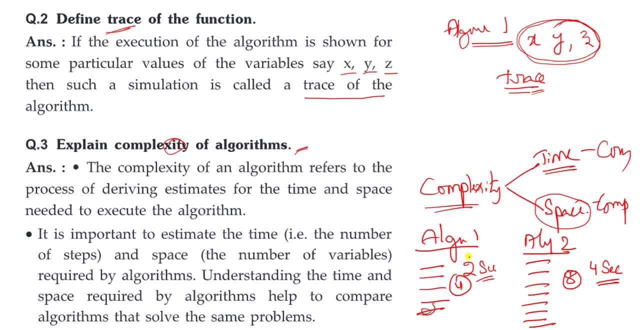 seconds. so uh, which one, which one is? algorithm one is the best one. algorithm two is the best one. uh is the best one. algorithm two is the best one. algorithm three is the best one. algorithm four is the best one. algorithm three is the best one. algorithm four is the best one. algorithm five is the best one. 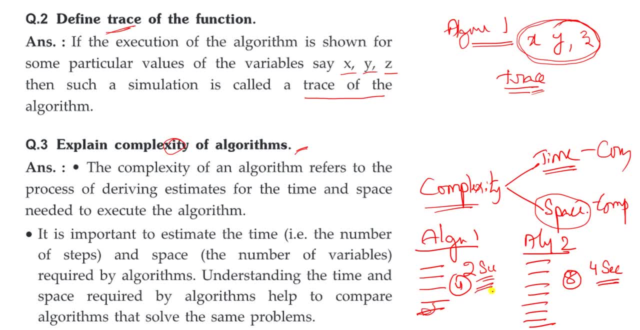 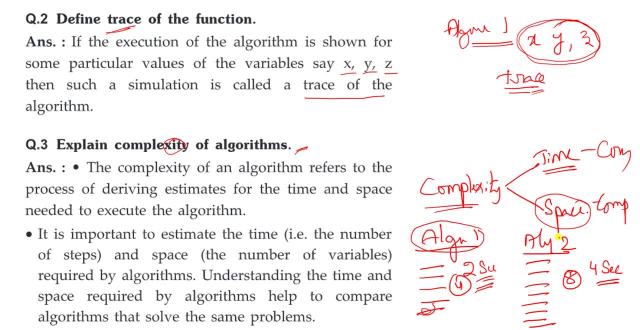 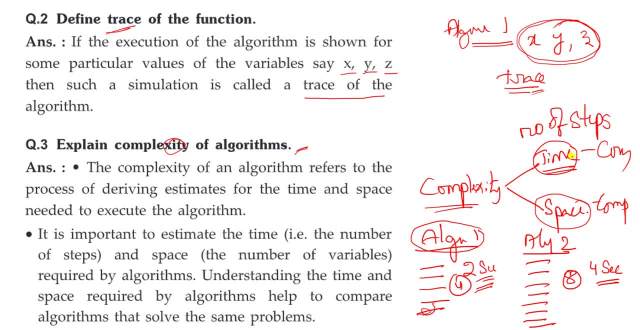 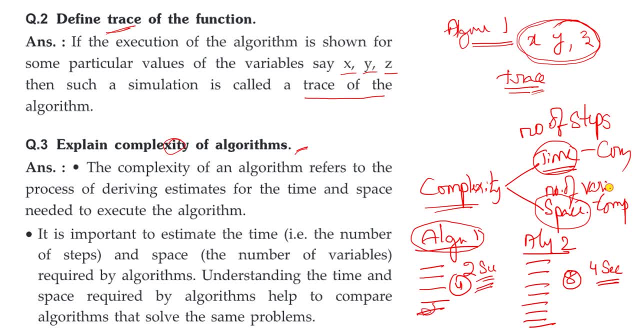 of number of variables. what do you mean by here, number of variables? so how many variables are required? this algorithm, for example, here we have only two variables, but here we have x, y, z, a, b, c. how many variables? 1, 2, 3, 4, 5, 6, 6 variables- is there here two variables? is there right? so space? 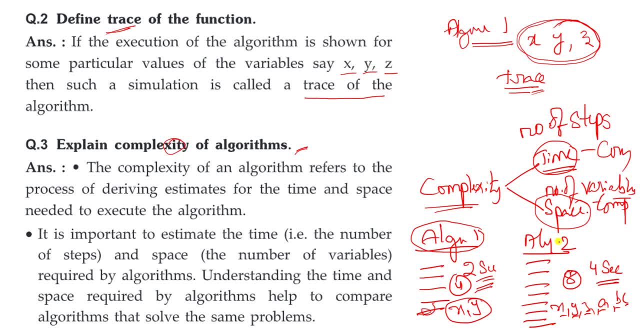 complexity, how we can estimate the space, how much space is required. you see we have some integers, float character, concept, right. so integer means two bytes. let us take some integer: x comma y, x comma y, two integers here. so we require only four bytes, only x comma y, two variables for this. 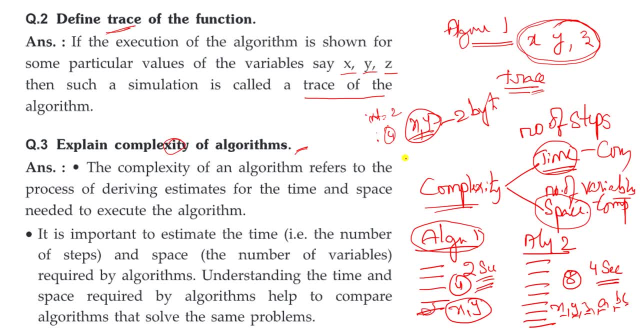 we required only two bytes. let us take okay, and the remaining x, y in algorithm 2? it requires how much space? for example, 10 bytes. okay, so which one? algorithm 1 requires two bytes. algorithm 2 requires only two bytes. so we require only two bytes for this. algorithm 2 requires only two bytes. 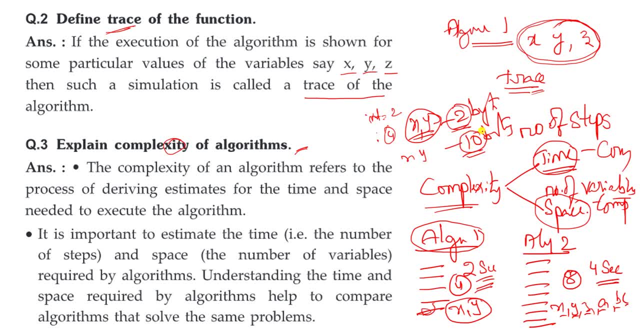 only 10 bytes. so which algorithm executes first? obviously two bytes algorithm executes first, then algorithm 2 will execute. hope you understand right. so here, understanding the time and space that is required by the algorithm, it will. it will help to compare the algorithms. so, based on this, 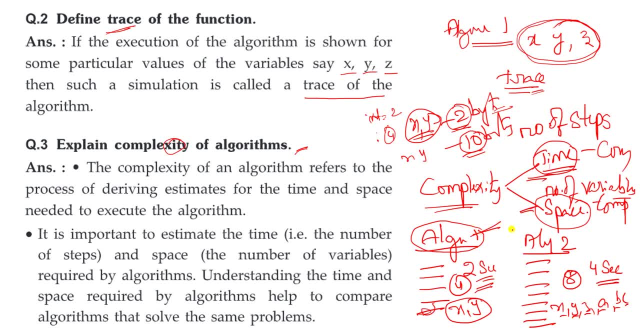 time. based on the space, we can compare this one, we can compare algorithm 1 and we can compare algorithm 2. here the steps is less so. execution time is less. so we can compare algorithm 1 and we can compare algorithm 2. here the steps is less so. execution time is less. here the number of variables is: 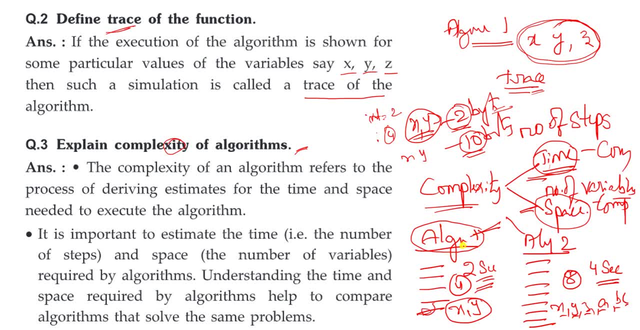 low. okay, number of variables is very less. so only two number, two number of variables is there. so here space also required. algorithm 1 requires less space for this particular two variables. but in case of algorithm 2 we have the two criteria, that is, time and space. okay, so algorithm 2- time requires. 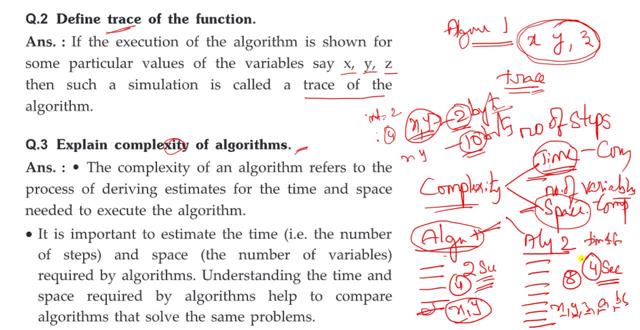 four seconds. four seconds so when compared to algorithm 2, it requires four seconds. so we can compare the algorithms. compared to algorithm 1, it 2 seconds more and also when compared to algorithm 1. here variables also more, ok, 6 variables will be there. so this is how we can compare the algorithms. 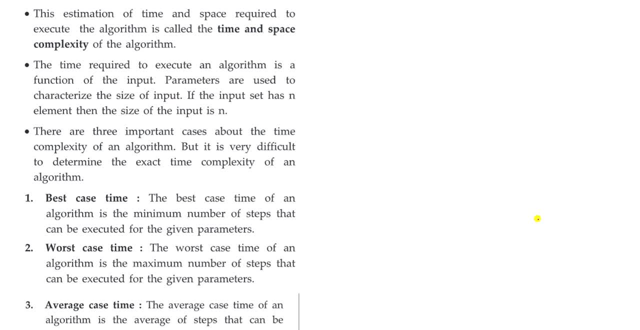 with the help of time and space. so the estimation of time and space requires the execution, the algorithm. in order to execute in particular algorithm, let us take some algorithm. so here we have some steps like x, comma, y, comma, z, ok, x equal to some value, value 1 and y is. 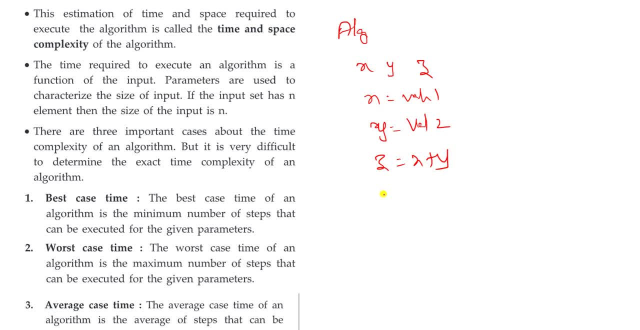 equal to value 2 and z is equal to x plus y and then print z. so how many steps we have? 1, 2, 3, 4, 5 steps. is there? ok? so the estimation time, the estimation of time and space. i told you already complexity, time complexity and space. complexity is very important, so here: 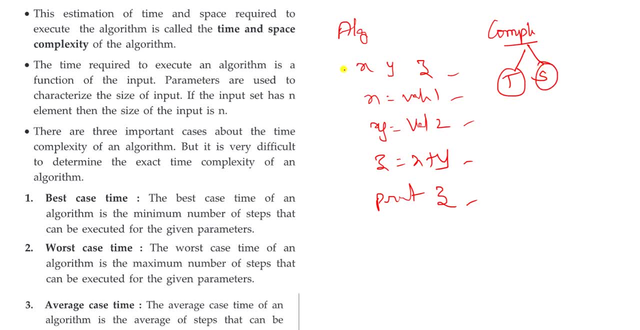 time and space Required to execute the particular algorithm. so, in order to execute this particular algorithm, what we required? we required time complexity and we required space complexity. time requires to execute an algorithm is a function of the input. ok, so here, what are the parameters we are used in this algorithm? that is nothing but size of the input. so here we can say that. 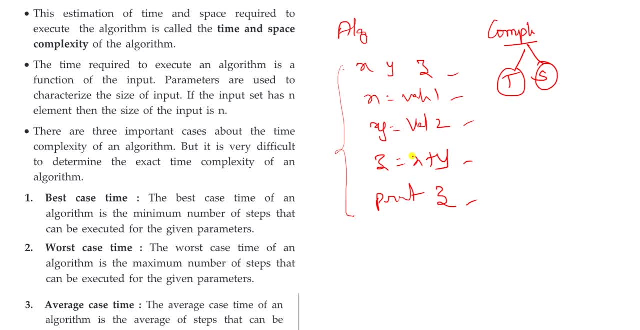 we. actually it is very difficult to determine the exact time complexity. we cannot determine the exact time complexity. We cannot determine the exact time complexity, but we there are some important cases will be there. that is, three important cases will be there in the complexity of algorithm. that 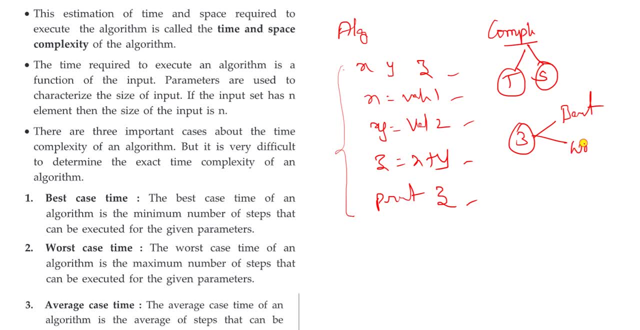 is best case time, best case and worst case and average, ok, average. so here we have: how many types of complexity of algorithm, how many types, how many cases in complexity of algorithm, First case time and also average case time. So best case time is nothing but an algorithm is minimum number of steps. 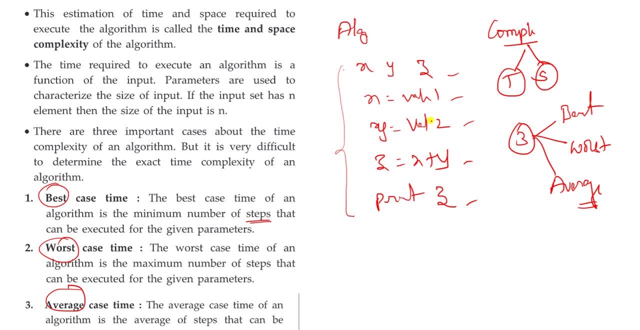 For example, minimum number of steps will be there. If the number of steps is less, then execution time is less, So that is the best case. If the number of steps is more, maximum number of steps is there in the algorithm. 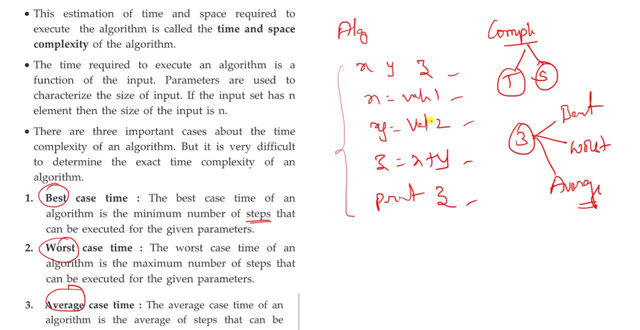 then automatically execution time automatically increases, Right, So here, just have a look. here. Number of steps is less Okay. I will indicate: the less is down arrow: Okay, Execution time is less Okay. If number of steps more, then automatically execution time is more. 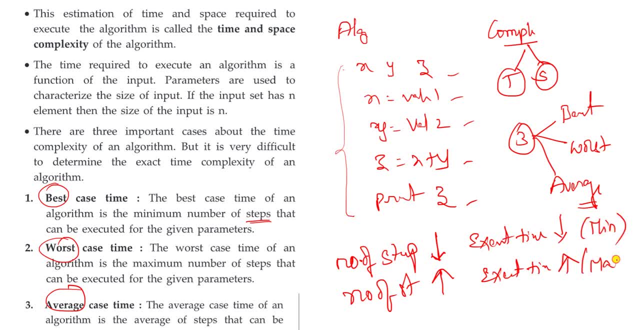 Okay, This is in the case minimum number of steps. It is in the case maximum number of the case. That is the thing here: Minimum number of steps. execution time is less. That is the best case. So this is the best case. 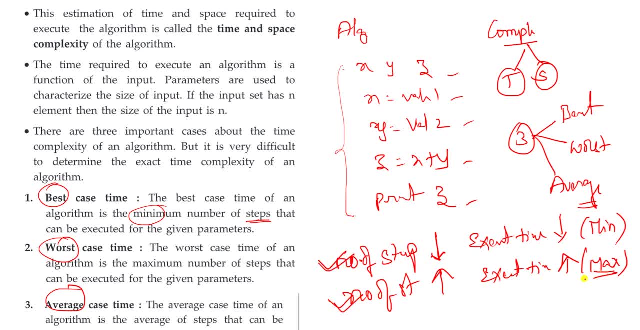 Now, this is the worst case. If the maximum number of steps will be there, then execution of time is more So. that is the worst case. What is the average case of time in an algorithm? Average steps that can be executed for the word. 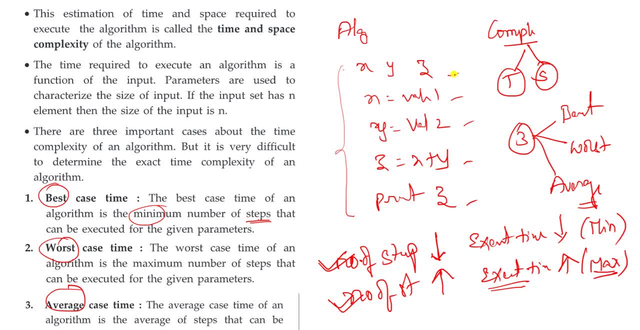 For example, average time means here, For example this particular algorithm, how much time we required to execute. Let us take some 2 minutes. Okay, Let us have some algorithm 2.. Okay, This particular algorithm have some 15, 50 steps. 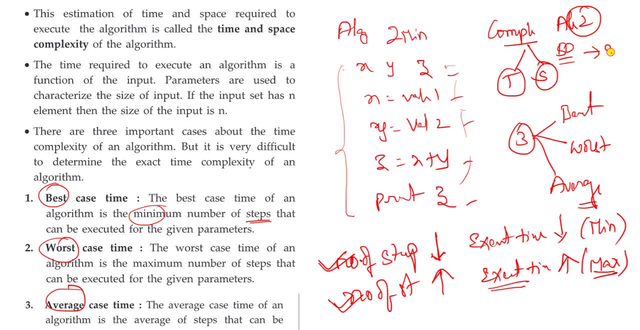 Okay, It requires Some 8 minutes time. Okay, Let us assume. Let us take the values 2 minutes and 8 minutes. So for algorithm 1, 2 minutes. For algorithm 2, 8 minutes. So what is the average case time for these 2 algorithms? 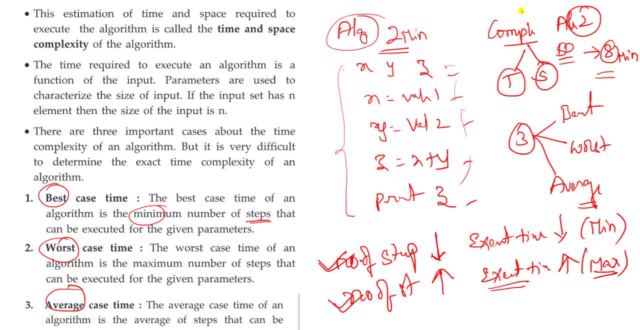 For what is the So in the time? So what is the average time In the time? So what is the average time Like 2 plus 8 by 2.. That is 10 by 2 in minutes of 5 minutes. 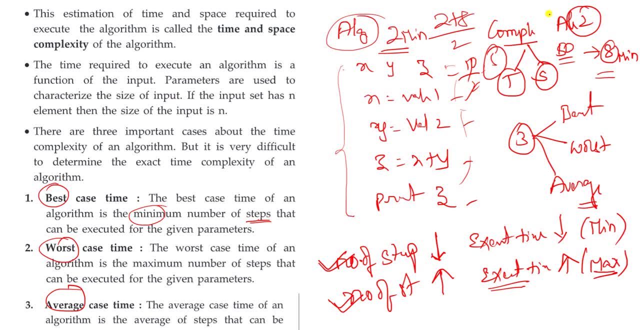 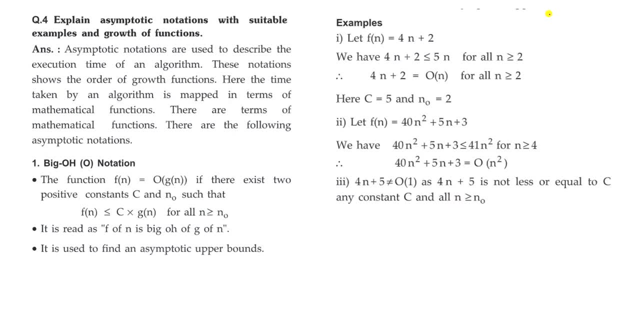 Okay, So average case here: 5 minutes. So that is about best case time, worst case time and average case time. So this is about complexity of algorithm. Very, very important. And next one And next important topic in algorithms is growth of the functions. 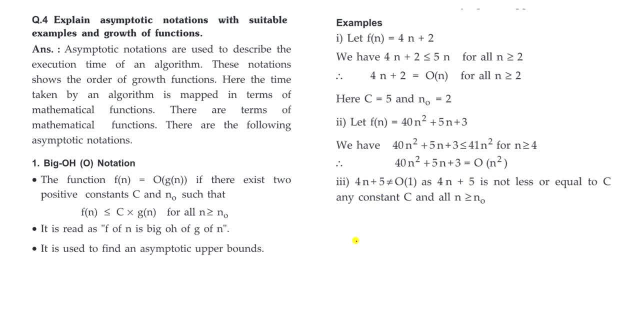 So how you can find out the growth of the functions means with the help of asymptotic notations. With the help of asymptotic notations we can find out growth of the functions. So here we can describe the execution type And 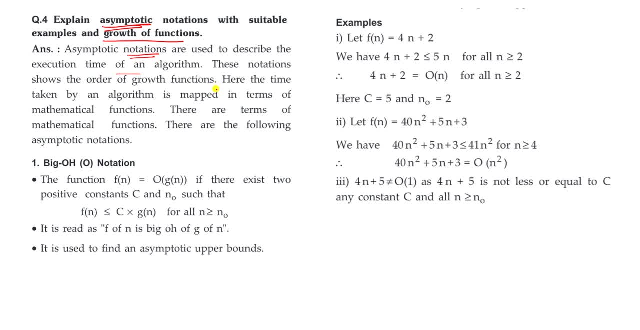 Execution time of algorithm with the help of these notations. So these notations shows the order of the growth functions. So here how much time is taken by an algorithm that is mapped in terms of the mathematical functions. So there are some mathematical functions we have. 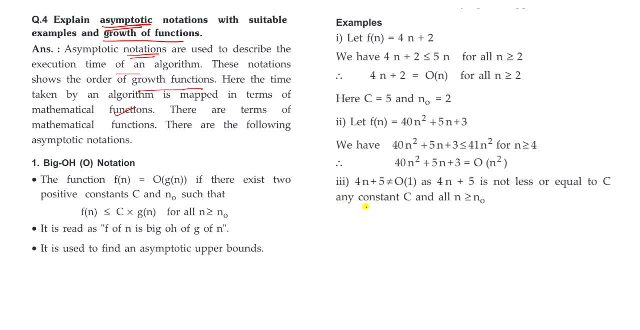 There are some asymptotic notations we have. So how many we have, That is 3.. Asymptotic notations means a n. Okay, So we have 3 ma. That is big O notation And Omega notation. 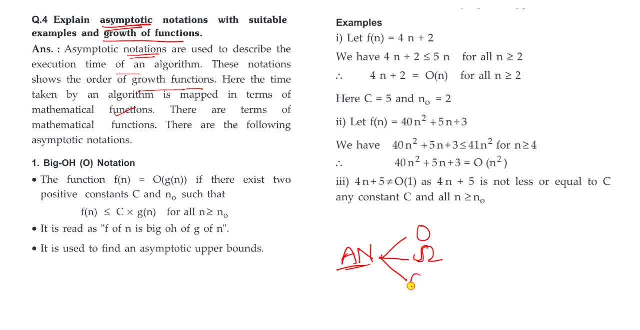 So this is called omega, Omega, this one Omega And next one theta notation. Okay, So we have big O notation, Big O, Right, We have to denote big O And this is sigma, Not sigma, This is omega. 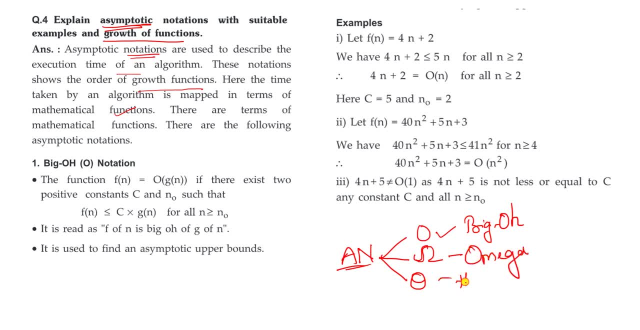 Omega, Omega notation, And this one is theta. You know this one, Theta. Okay, So what do you mean by big O notation? How we can estimate time, execution time of algorithm with the help of big O notation. How we can estimate the time of our growth of an algorithm with the help of big O notation. 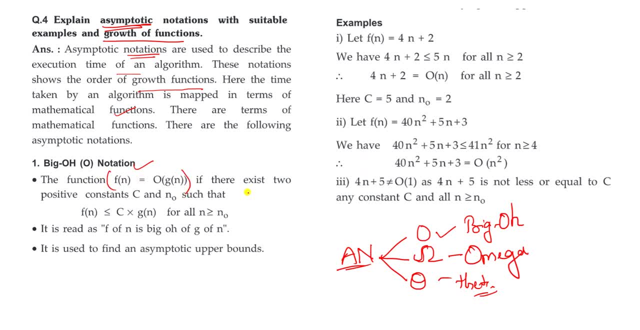 Right. So here how we can denote the function: f of n is equal to O of z of n. So how we can denote f of n equal to O of big O, Big O of z of n here. So the main thing here. 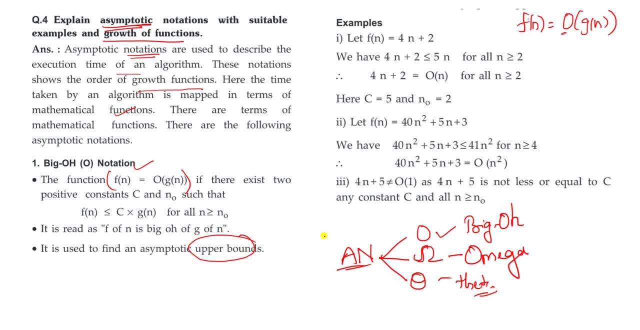 It is used to find the upper bounds. only Big O notation find out upper bounds, Okay, And similarly omega will have to find lower bounds, Lower bounds. Do you know upper bound and lower bounds? Let us take some example, like 16,, 17,, 18.. 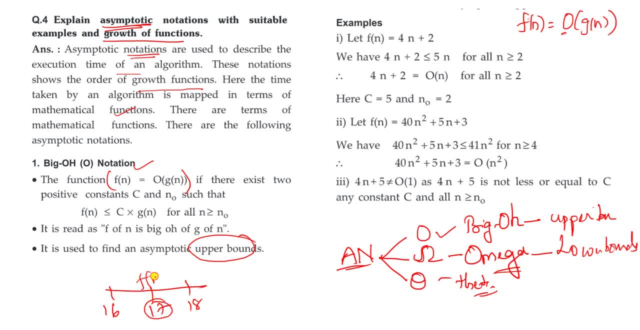 Okay, Here the middle number is, Let us take this is the f of n. Okay, So what is the upper bound of 17?? That is this one. So after 16,, after 17 and 18, we have: 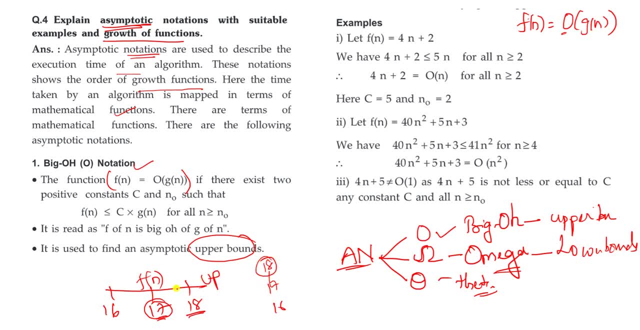 So upper bound is what 18.. So this is upper bound and the 16 is lower bound. Clear. So in order to find out this upper bound, what we have to use Big O notation. In order to find out the lower bound, what we have to use. 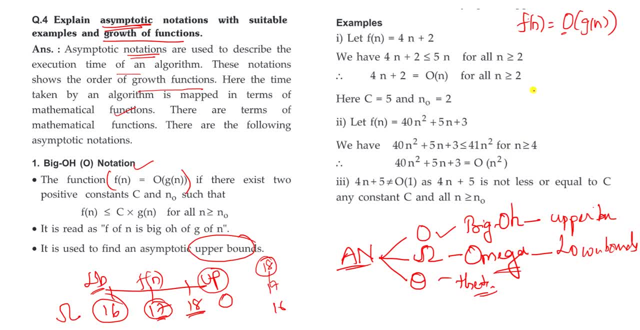 Omega. Okay, That is the thing here. Let us take another example like 36,, 37,, 38. Just assume: Okay, Okay, So what is? So what is the upper bound here? 38. So let us take: f of n is 37.. 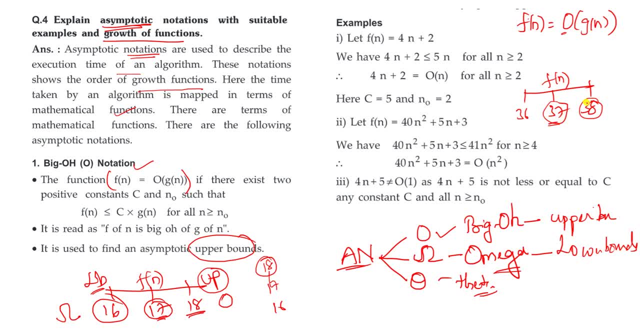 Let us take f of n is 37.. So what is the upper bound of 37? That is 38.. What is the lower bound of 37? That is 36.. This is the lower bound. So in order to find out this upper bound, what we have to use the notation. 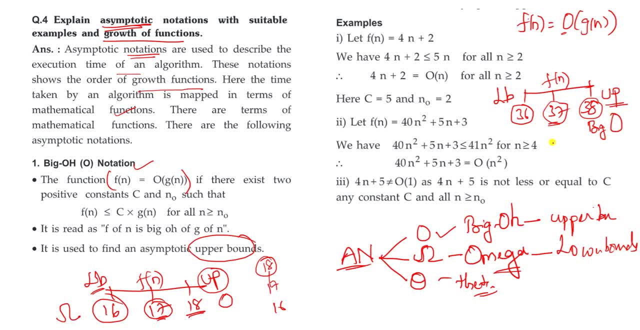 Big O notation, What we have to use. Big O notation: Okay, So, in order to find out the lower bound of 37.. Here we have to Tell: upper bound of 37, lower bound of 37.. Okay, So, in order to find out the lower bound of 37, what we have to use. 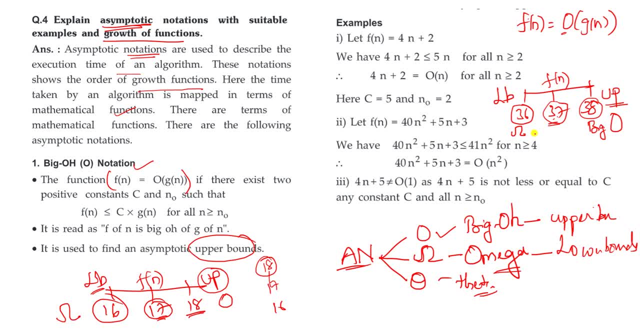 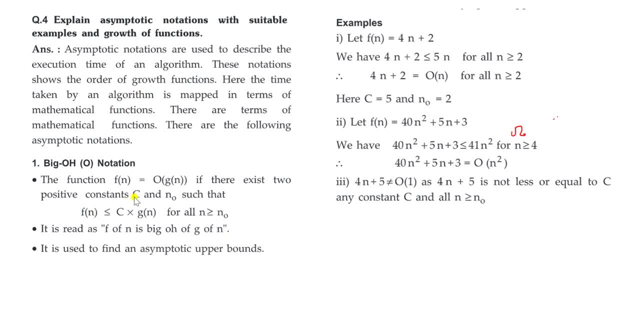 Omega, Omega g of n Clear. So how it will be, See the function constant, here The existing positive constants, That is, c and n naught. c and n? naught such that f of n is less than or equal to. 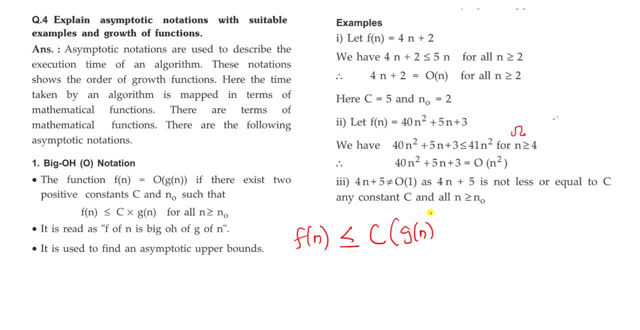 c, of c, of g, of n. Okay, Here we have to find out upper bound. This is upper bound value, So it should be lower value, Like man: 36,, 37, 38. No, So anyhow, 37 is less than 38.. 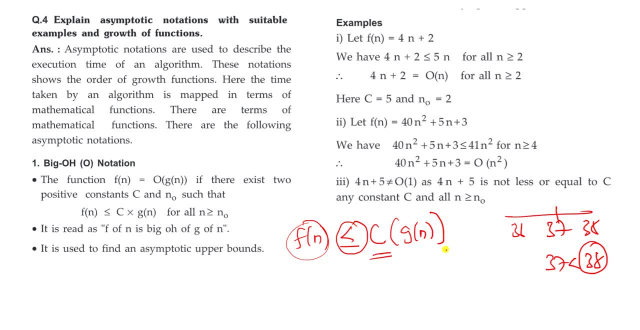 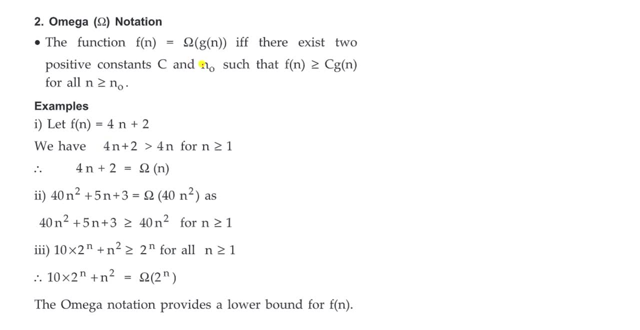 Right. So this is the upper bound value, So it should be always less than or equal to In case of omega. Let us take, in case of omega, What we have Greater than or equal to Clear. So f of n is greater than or equal to. 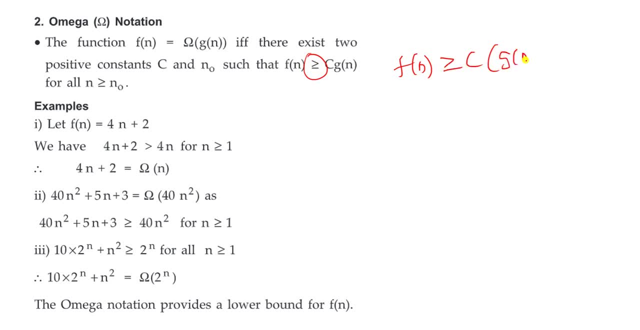 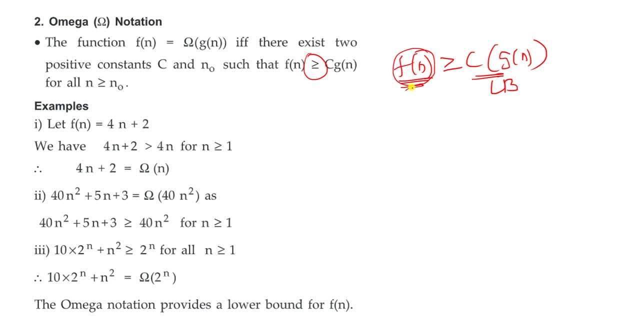 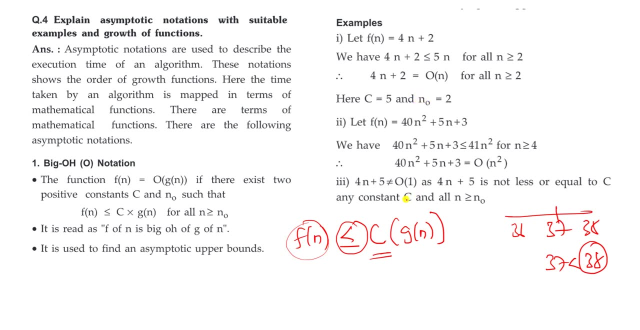 Okay, Here we need to find out lower bound of f of n, So it should be in greater than or equal to. So this notation is very, very important, students. Okay, f of 1, less than or equal to c of g of n. 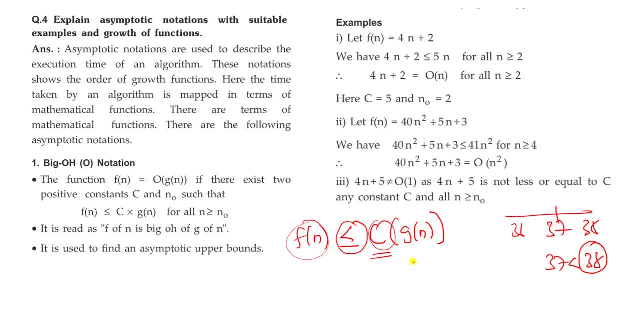 Here c is a constant and n is also constant, Okay. Here we have a two positive constants, That is, c is a constant, Okay, And n, naught of g, of n, is also a constant, or n1 is a constant, clear. So what we have to remember here: exam point of view: big O is used. 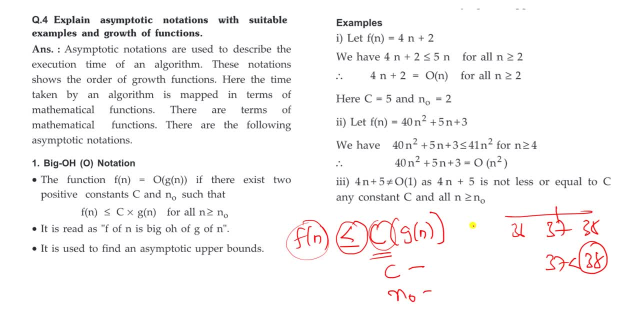 for, assume, find out the upper bound of a particular function. ok, Omega is used for to find out the lower bound of a particular function. ok, See the example: 4n plus 2 and we have the notation 5n. ok, So here the function f of n is equal to 4n plus 2, right? So 4n plus 2, less than or equal. 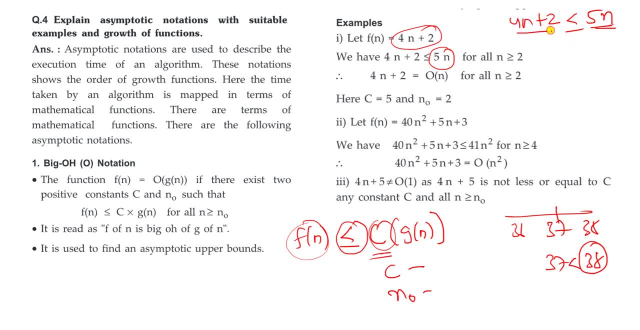 to 5n. So here, this is the upper bound, this is the f of n, this is the f of n less than or equal. this is the upper bound. So that means c of g of n. ok, So what is the c here? 5, clear. So. 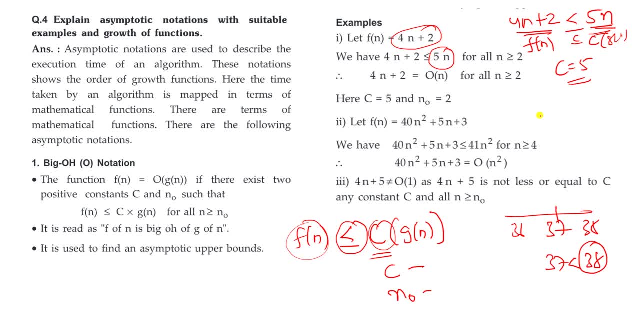 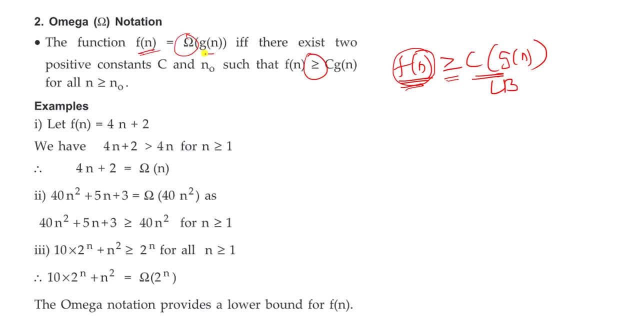 like this we have to do the sums. Next one: omega notation. So in omega notation, function n, that is omega g of n, where existing positive constant c and n naught, it should be greater than or equal to Simply the negative of big O notation, that is, omega ok f of n. it should be greater than or equal to g of n. So this is the. 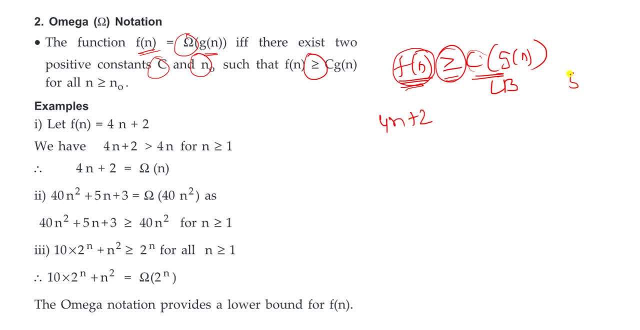 lower bound. For example, 4n plus 2, 5n. 5n is greater than ok, just, and what will be the less? than So here, 4n plus 2 is less than 5n, ok. So this is the upper bound value, this is the lower. 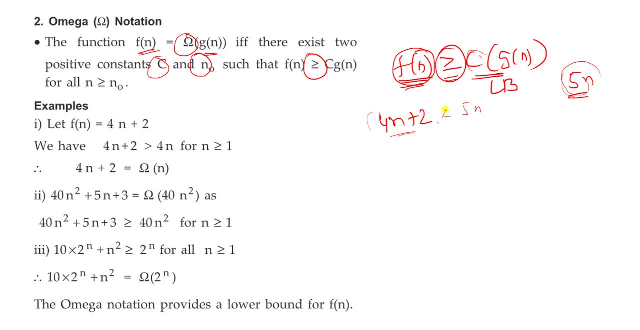 bound value. So what is the lower bound of this value? that is 4n. Let us take, let us assume 4n. Let us simple: n equal to 1. take n equal to 1, ok, So 4 into 1 plus. 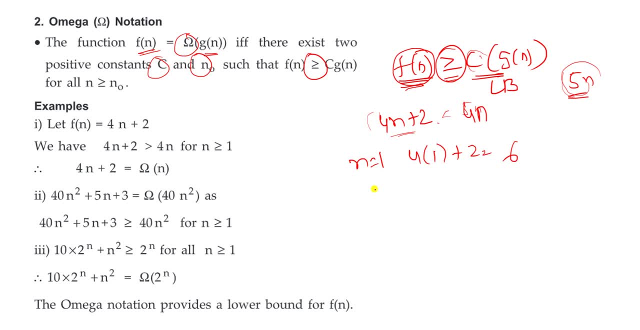 2, that is 4 plus 2. for ones of 4,, 4 plus 2, 6. ok, and here 4n n equal to 1, 4n 4 into 1, 4.. So which one is greater than this? one is greater than 6 is greater than 4, right? So 4n plus 2, greater than. 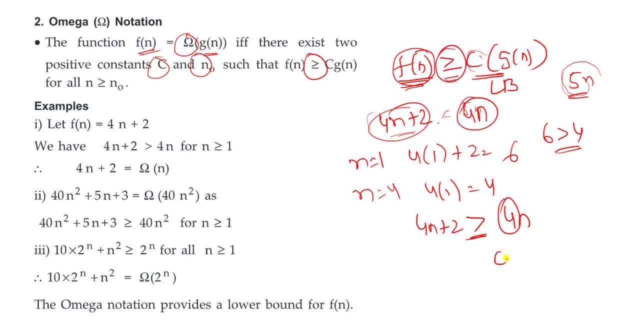 we have to assume greater than or equal to 4n. So here c is equal to what 4 n naught is greater than or equal to what n clear. So like this we have to do In the second example, also 40 n square 5n. 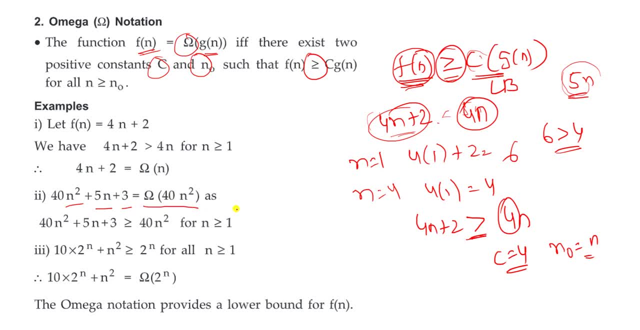 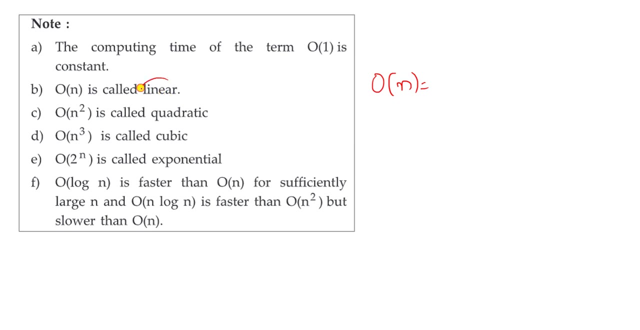 plus 3 sigma what he gave 40 n square right. So here 40 is the c, c is equal to 40.. Now some notations. we have, for example, o of n, o of n. that is called a linear If o of n is there. 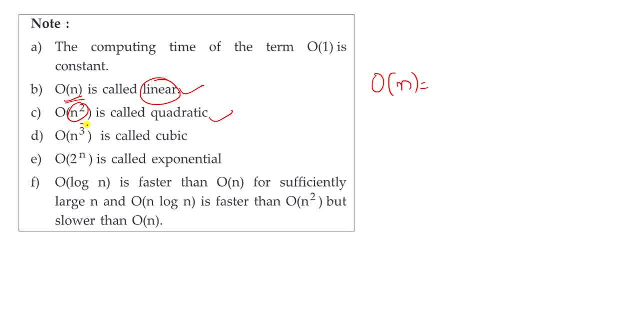 it is linear. n square is there, that is quadratic. If n cube is there, that is cubic. If 2 power n, 2 power n is there, that is exponential. ok, and logarithms. you know the logarithms: right O of log n is faster than is faster than whom? o comma n. 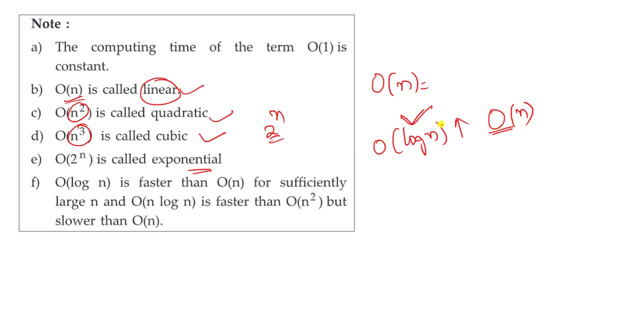 o of n, o of n- this one is faster, ok, and for sufficiently larger n and o of n log n is faster than o of n square. Remember this point, you may get, You may, whatever AB I say here Today. you are saying a two stage problem. That means 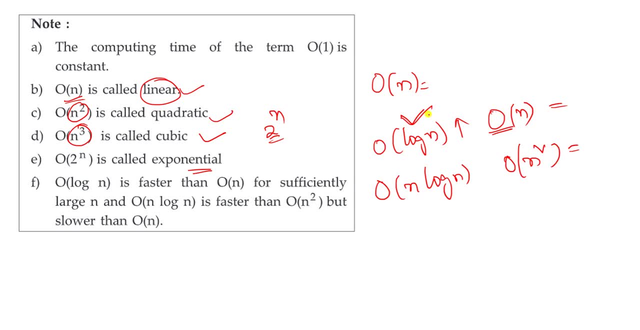 we have given q3. you can find the jitive example, which is: a: n equals c plus x, square root n power n in. Now we are from N 3, N 2 here, right. So which juntPHx to N 1 그런데? 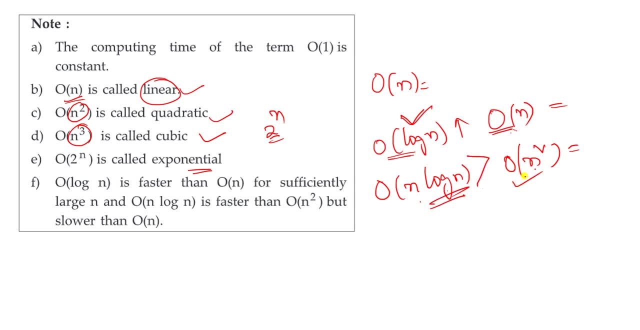 you write this c to the right, who stand on the denominator and square root, n, sometimes equal 0, 0.. Anyway, n is right in d, z is vd-f. 3 will give equal into n plus x plus x square n d. It is a power thing. How long will be the table? Yes, When you take .22.. Just drink. 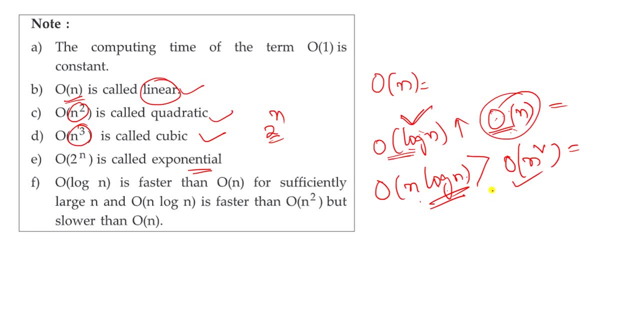 it and come in and learn This process of relationship. cold engine problems. the Waltz is best I have to: o of log n, o of n? o of n log n. low. o of log n, when compared to o of n. first, when compared to these, 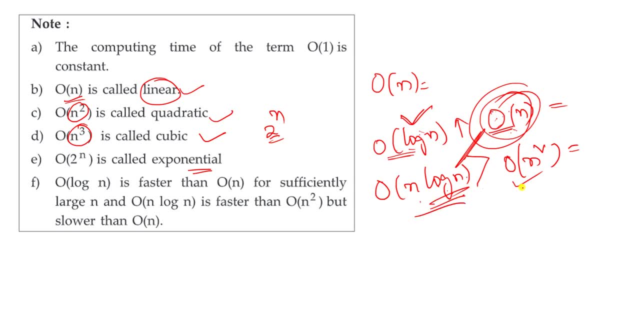 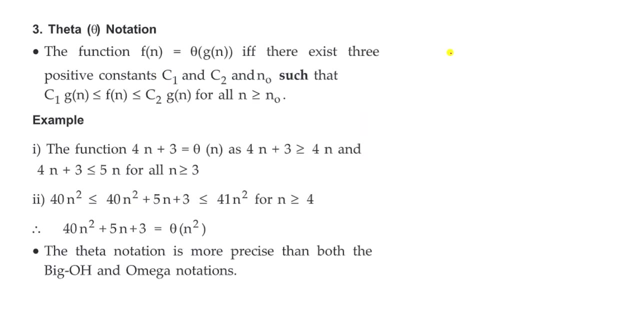 two. this one is good, clear when compared to these two. this one is good when compared to these two, this one is good. so here they are, like like this: we have to find out. and the last one: theta notation. theta notation means between the value, so here we find out, upper bound value and lower. 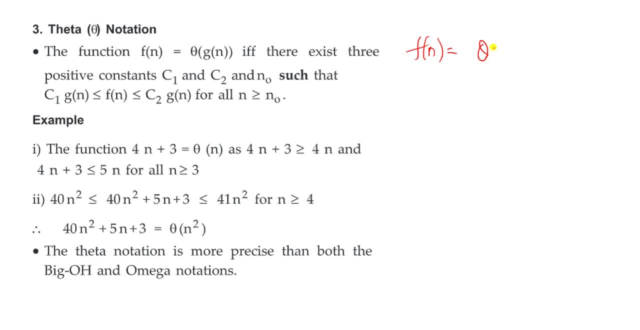 bound value. so here f of n equal to theta, g of n, theta of g of n. so f of n less than or equal to big, o, g of n, f of n greater than or equal to omega and f of n equal to theta. okay, so here theta is. 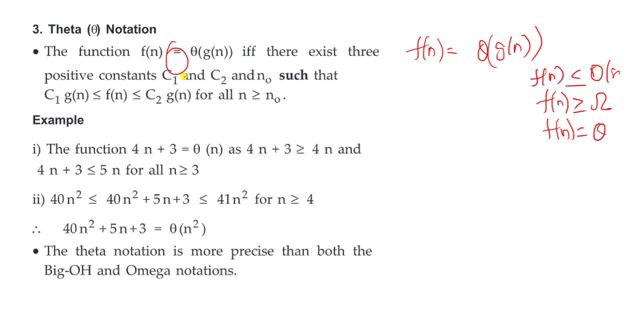 so what we have to do here, we have to take two constants, c 1 and c 2, and n naught. so c 1 g of n, less than or equal to f of n, less than or equal to c 2 g of n. so simply here, let us take some 55. 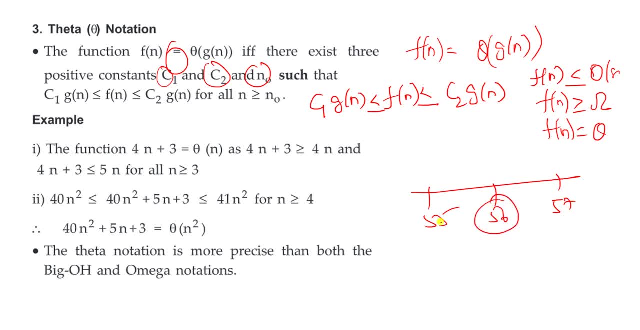 56, 57. okay, so 55 is less than, 56 is less than 57, so this is the theta notation. this is the theta notation. likewise, 12, 13, 14. okay, 12, less than 13, less than 14, so this is a theta notation. 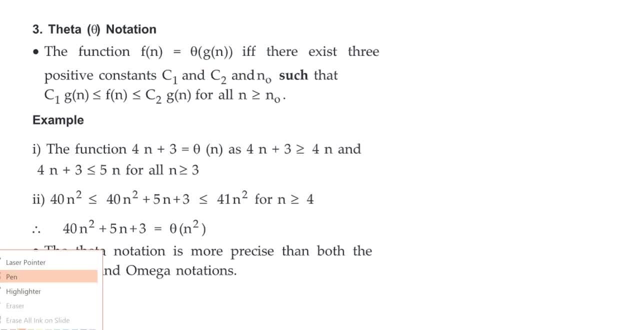 likewise, see the example here um the function 4n plus 3 equal to theta. so what is the function? 4n plus 3 is equal to theta, so 4n plus 3 is greater than or equal to 4n. greater than means what it is.